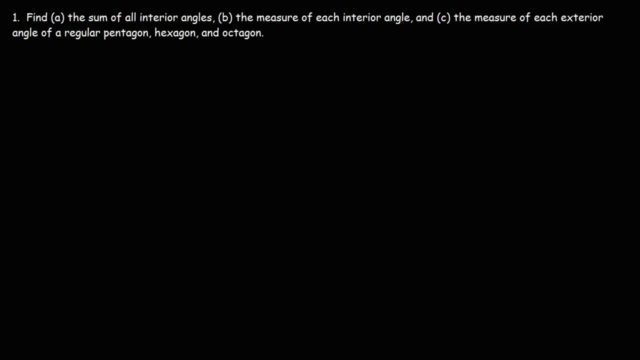 In this video, we're going to talk about how to calculate the measure of the interior angle of a regular polygon, and also the exterior angle as well. So let's start with the pentagon. A pentagon is a polygon with five sides. Now, because we're dealing with a regular pentagon, all sides are equal and all of the interior angles are the same. 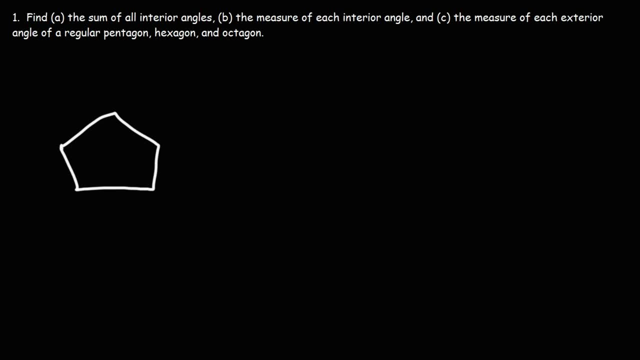 Now we want to find the sum of all of the interior angles. So, by the way, this is the interior angle And here, if we extend one of the sides, we can get the exterior angle. Notice that these two angles, they form a linear pair. 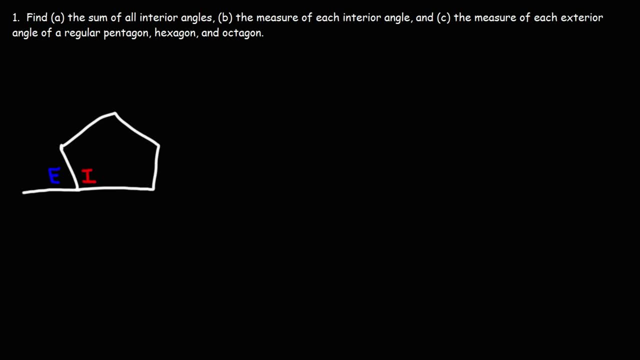 So they must add up to 180.. Now to calculate the sum of the interior angles, it's simply 180 times n minus 2, where n is the number of sides on the polygon. So the word penta means 5.. 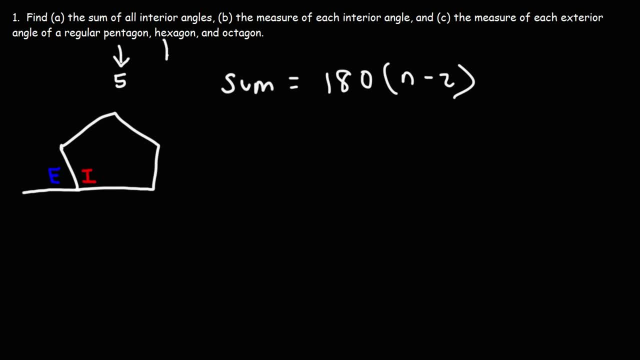 So we're dealing with a five-sided polygon. Hexa represents 6.. Octa is 8.. So tri triangle, that's a three-sided polygon. Quad means 4, quadrilateral, four-sided polygon, A heptagon. hepta means 7.. 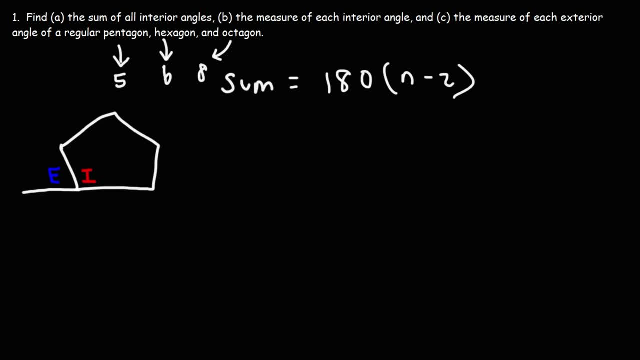 Nana is 9.. Deca is 10.. But for this one we're dealing with a pentagon, so n is 5.. Now, 5 minus 2 is 3.. 180 times 3 is 540.. 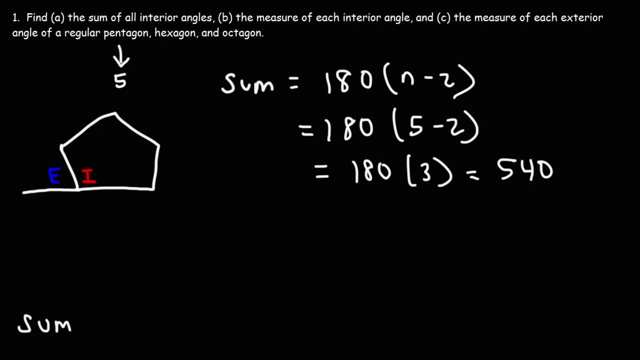 So for a regular pentagon, the sum of all of the interior angles is 540 degrees. Now let's move on to part B. Let's calculate the measure of each interior angle. To find the measure of each interior angle, we could take the sum of all the angles and divide it by n. 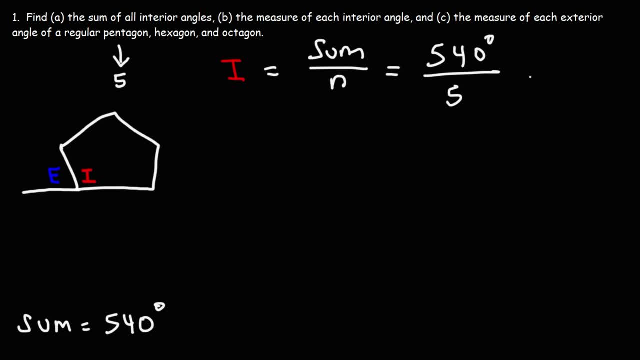 So it's 540 degrees divided by the five sides. And if you want to do this mentally, see it this way- You could break 540 into 500 plus 40. And then divide each by 5.. So 500 divided by 5 is 100.. 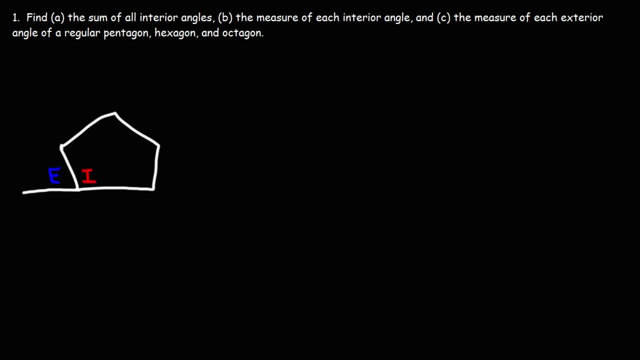 So they must add up to 180.. Now to calculate the sum of the interior angles, it simply 180 times n minus 2, where n is the number of sides on the polygon. So the word penta means five. So we're dealing with a five-sided polygon. 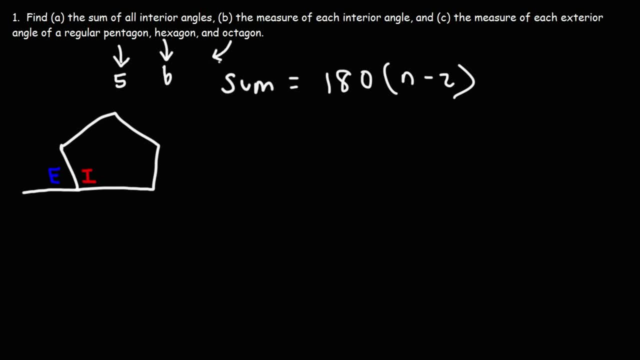 Hexa represents six, Octa is eight, So tri triangle, that's a three-sided polygon. Quad means four, quadrilateral four-sided polygon, A heptagon. hepta means seven, Nana is nine, Deca is ten. 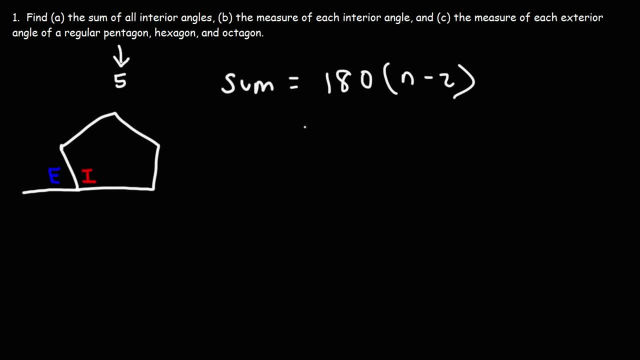 But for this one we're dealing with a pentagon. so n is five. Now, five minus two is three. 180 times three is 540.. So for a regular pentagon the sum of all of the interior angles is 540 degrees. 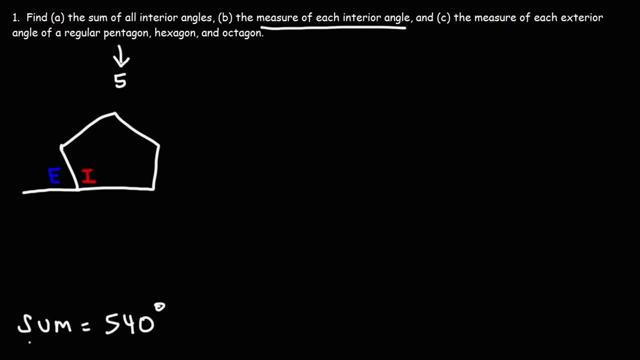 Now let's move on to part B. Let's calculate the measure of each interior angle. To find the measure of each interior angle, we could take the sum of all the angles and divide it by n. So it's 540 degrees divided by the five sides. 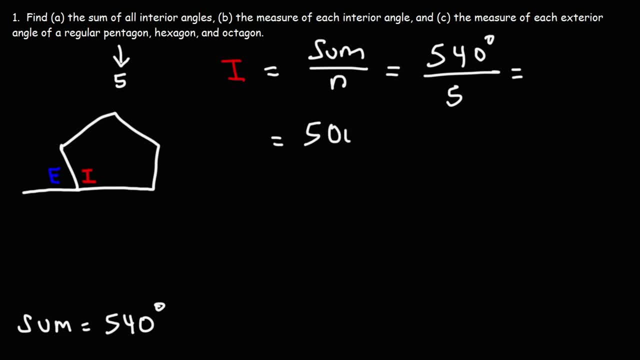 And if you want to do this mentally, see it this way, You could break 540 into 500 plus 40 and then divide each by five. So 500 divided by five is 100.. 40 divided by five is eight. So the measure of each interior angle is 108 for a regular pentagon. 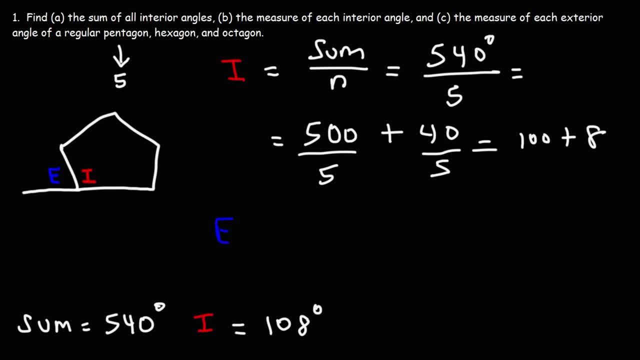 Now let's calculate the exterior angle. There's two ways in which we can do it. So, because the interior and the exterior angles are supplementary, that means that they add up to 180.. So the exterior angle is simply 180 minus the interior angle. 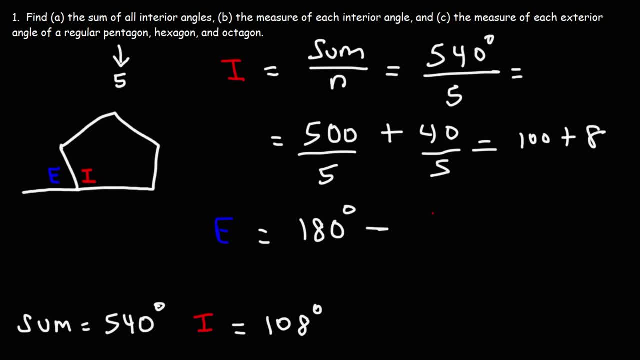 So the exterior angle is simply 180 minus the interior angle. So the exterior angle is simply 180 minus the interior angle. So the interior angle is simply 180 minus the interior angle. So the interior angle is simply 180 minus the interior angle. 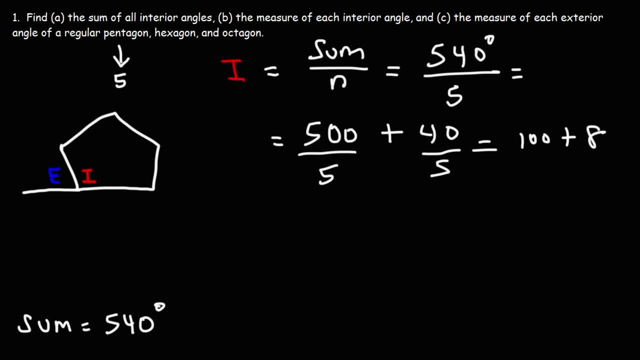 40 divided by 5 is 8.. So the measure of each interior angle is 108 for a regular pentagon. Now let's calculate the exterior angle. There's two ways in which we can do it. So because the interior and the exterior angles are supplementary. 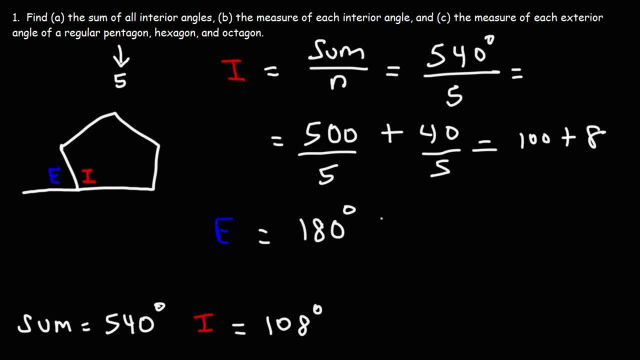 that means that they add up to 180.. So the exterior angle is simply 180 minus the interior angle, So that's 180 minus 108.. And that will give us 72 degrees. Now there's another way in which we can get the same answer. 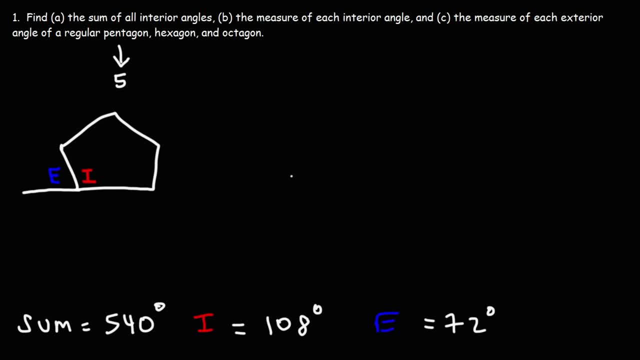 The measure of each exterior angle is simply 360 degrees divided by n, the number of sides of the regular polygon. So it's 360 divided by 5.. If you take 360 divided by 5, you'll get 72.. If you want to get the same answer, you can do it by dividing by 5.. 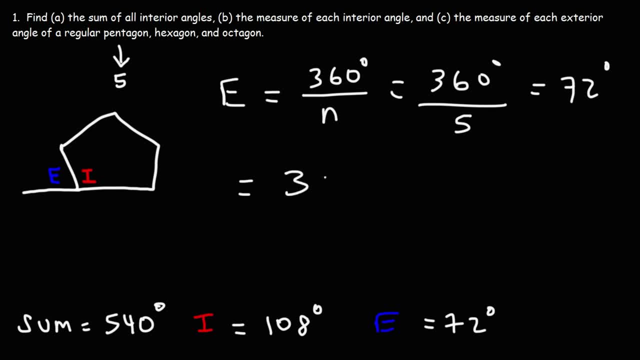 If you want to get that answer mentally, I would do it this way: I would break up 360 into 350 and 10.. 350 divided by 5. If you think of 35 divided by 5, that's 7.. 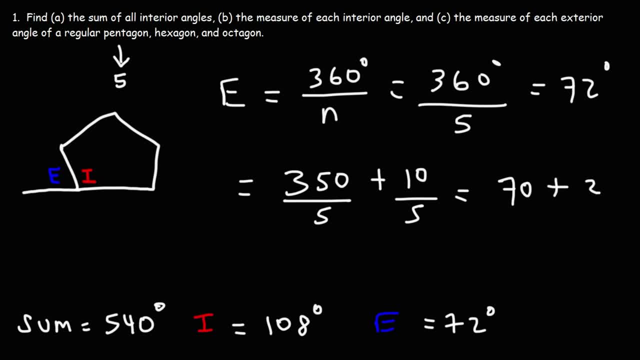 So if you add a 0 to that, you get 70. And 10 divided by 5, you get 2. So you get 72.. Now let's move on to the next polygon. Let's do the same thing for a hexagon. 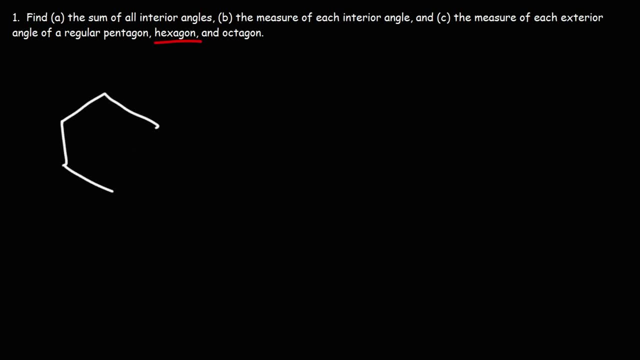 So let's draw a picture first. So there is our hexagon and we have six sides, And let's extend one of the sides, So we'll extend this side here. So we need to calculate the measure of the interior angle and the exterior angle. 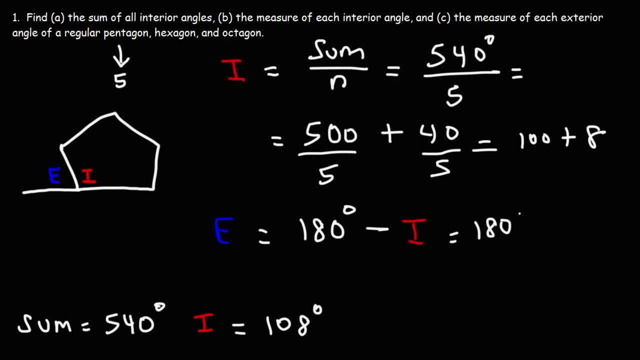 So the interior angle is simply 180 minus the interior angle, So that's 180 minus 108. And that will give us 72 degrees. Now there's another way in which we can get the same answer. The measure of each exterior angle is simply 360 degrees divided by n, the 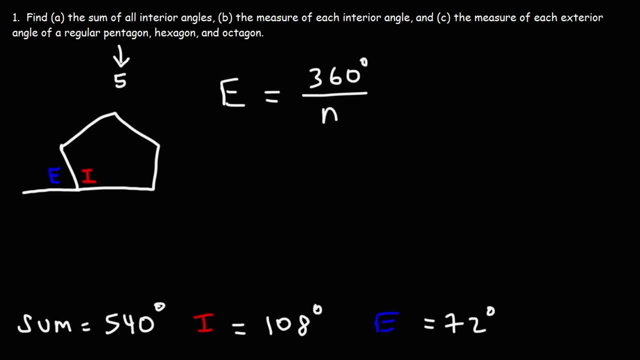 number of sides of the regular polygon. So it's 360 divided by 5.. If you take 360 divided by 5, you'll get 72.. If you want to get that answer mentally, I would do it this way. I would break up 360 into 350 and 10.. 350 divided by 5.. If you 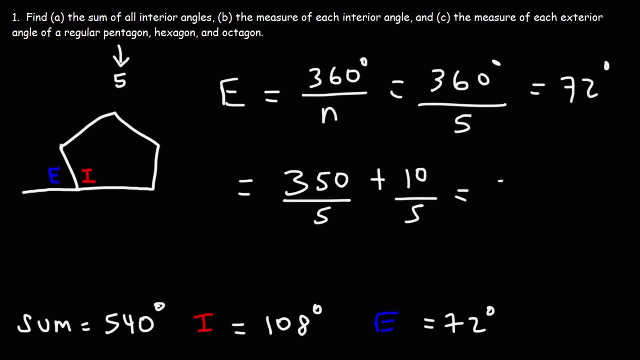 think of 35 divided by 5, that's 7.. So if you add a 0 to that, you get 70. And 10 divided by 5, you get 2. So you get 72.. Now let's move on to the next polygon. 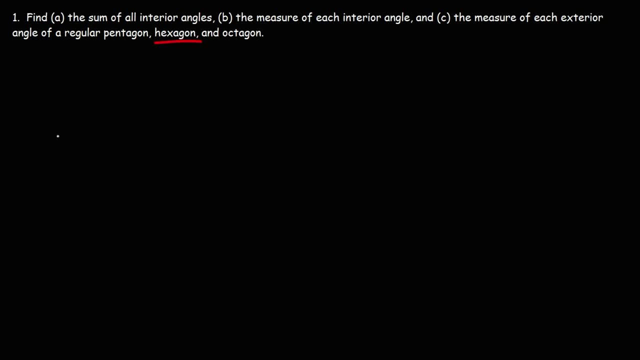 Let's do the same thing for a hexagon. So let's do the same thing for a hexagon. So let's do the same thing for a hexagon. So let's draw a picture first. So there is our hexagon, and we have six sides. 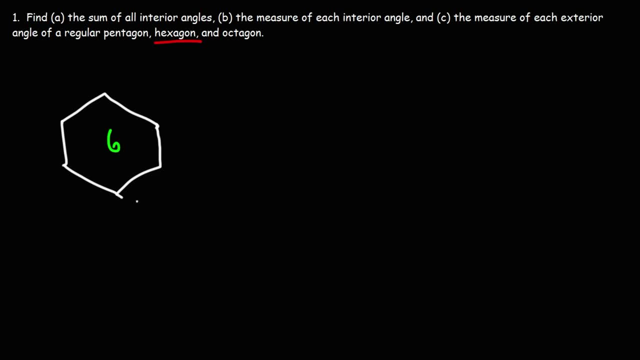 And let's extend one of the sides, So we'll extend this side here. So we need to calculate the measure of the interior angle and the exterior angle. So first let's calculate the sum. The sum is going to be 180 times n minus 2.. 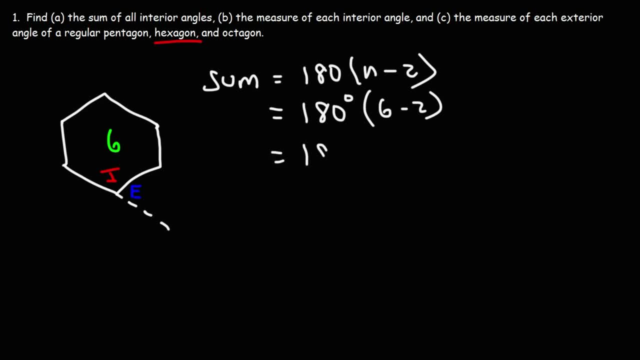 n is 6, so this becomes 180 times 6 minus 2, which is 4.. 18 times 4 is 72, so if we add the 0, we get 720 degrees. So that is the sum of all of the interior angles inside a regular hexagon. 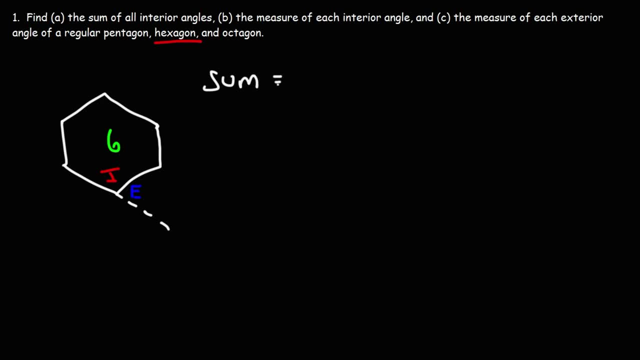 So first let's calculate the sum. The sum is going to be 180 times n minus 2.. n is 6.. So this becomes 180 times 6 minus 2, which is 4.. 18 times 4 is 72.. 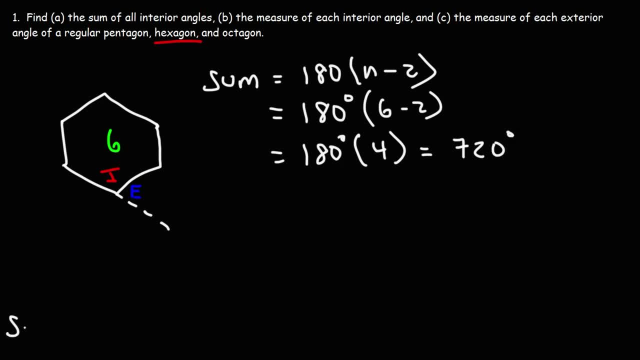 So if we add the 0, we get 720 degrees. So that is the sum of all of the interior angles inside, And the sum of all of the interior angles inside is a regular hexagon. Now let's calculate the measure of each interior angle. 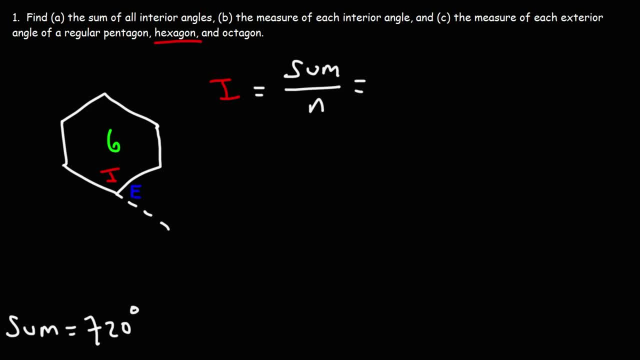 So it's going to be the sum divided by n, So it's 720 degrees divided by 6.. 72 divided by 6 is 12.. Add the 0,, we get 120.. So that is the measure of each interior angle. 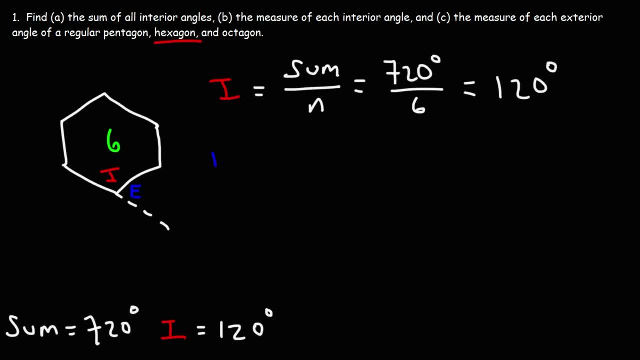 And we know these two form a linear pair And we know that the sum of all of the interior angles inside is a regular hexagon. So to calculate the measure of each exterior angle, it's going to be 180 minus 120, which is 60.. 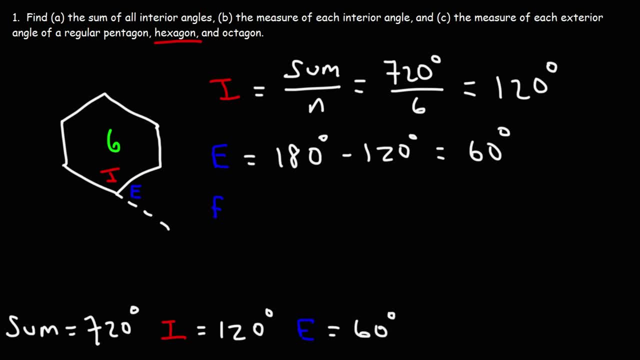 Now let's confirm that we do have the right answer. We know the measure of each exterior angle of a polygon is going to be 360 divided by n. So it's 360 divided by the six sides. 36 divided by 6 is 6.. Add the 0, we get 60.. So that's it for the regular hexagon. The sum of all of the interior angles is 720.. The measure of each interior angle is 120, and the measure of each exterior angle is 60.. Now let's move on to the next shape, the octagon. 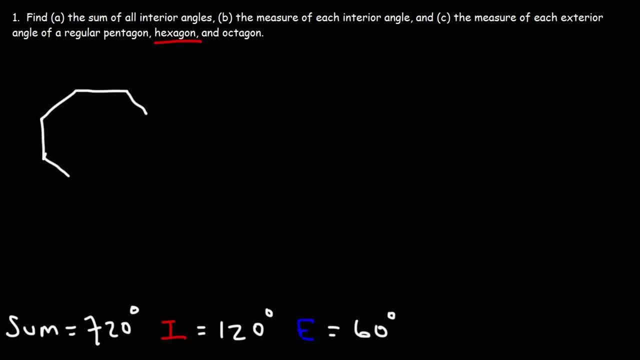 So the octagon has eight sides. That's how we can draw it, And here is one of the eight interior angles, And if we expand this side, here will be the exterior angle and the two of them will form a linear pair, as always. 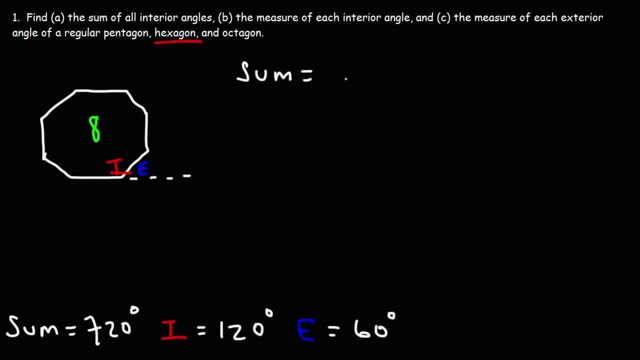 So first let's calculate the sum, The sum of all of the angles. It's going to be 180 times n minus 2.. n is 8, so this becomes 180 times 6.. And let's use a calculator for that. 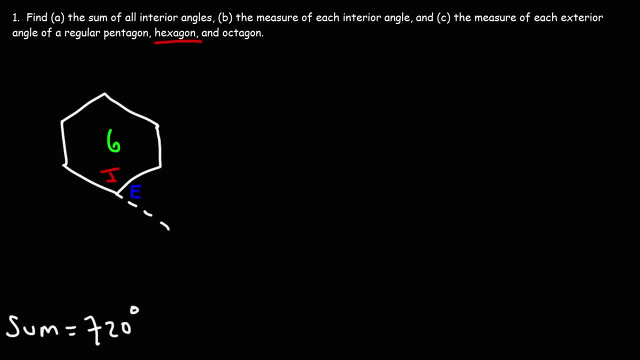 Now let's calculate the measure of each interior angle. So it's going to be the sum divided by n. So it's 720 degrees divided by 6.. 72 divided by 6 is 12.. Add the 0,, we get 120. 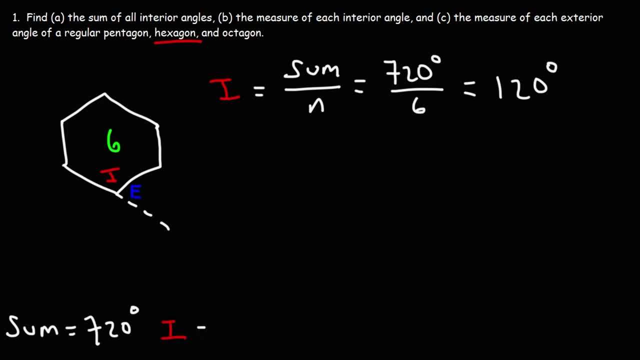 So that is the measure of each interior angle. And we know these two form a linear pair. So to calculate the measure of each interior angle, we need to calculate the sum divided by n. So to calculate the measure of each exterior angle, it's going to be 180 minus 120, which is 60. 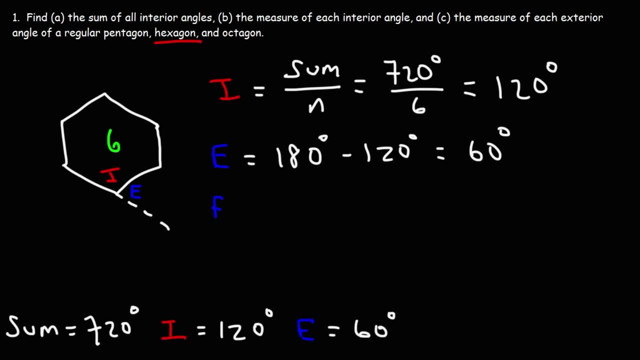 Now let's confirm that we do have the right answer. We know the measure of each exterior angle of a polygon is going to be 360 divided by n. So it's 360.. So it's 60 divided by the 6 sides. 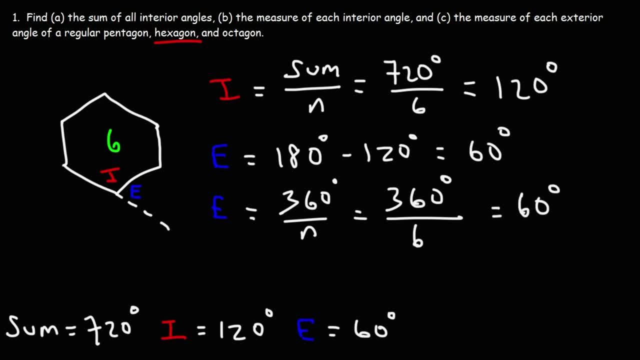 36 divided by 6 is 6.. Add the 0,, we get 60.. So that's it for the regular hexagon. The sum of all of the interior angles is 720.. The measure of each interior angle is 120.. 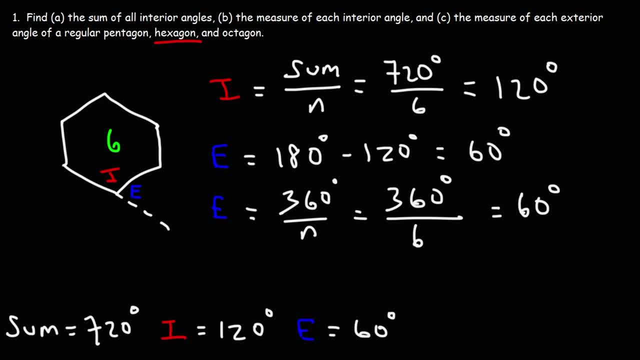 And the measure of each exterior angle is 60.. Now let's move on to the next shape, the octagon. So the octagon has 8 sides. That's how we can draw it, And here is one of the 8 interior angles. 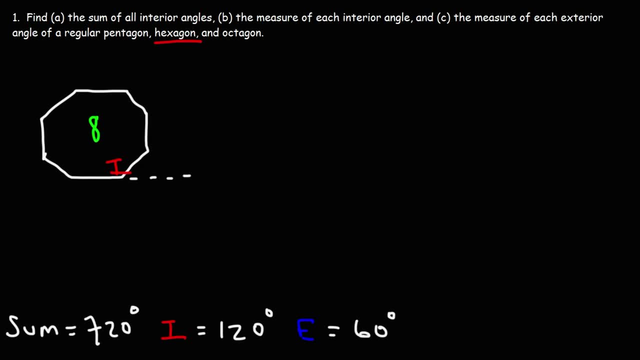 And if we expand this side, here will be the exterior angle, And the two of them will form a linear pair, as always. So first let's calculate the sum of all of the angles. It's going to be 180 times n minus 2.. 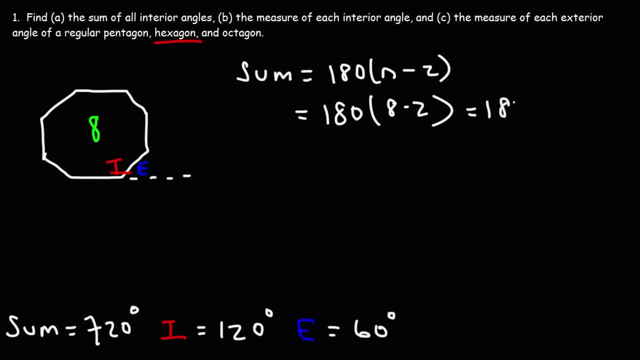 n is 8,, so this becomes 180 times 6.. And let's use a calculator for that. So 180 times 6.. 180 times 6.. Thus, the sum of all of the interior angles Is 1080.. 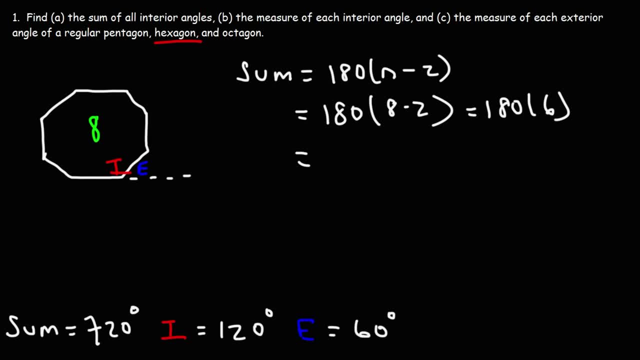 So 180 times 6.. Thus the sum of all of The interior angles is 1080.. Now to calculate the measure of each interior angle, it's going to be the sum divided by n, So that's 1080 degrees divided by the eight sides. 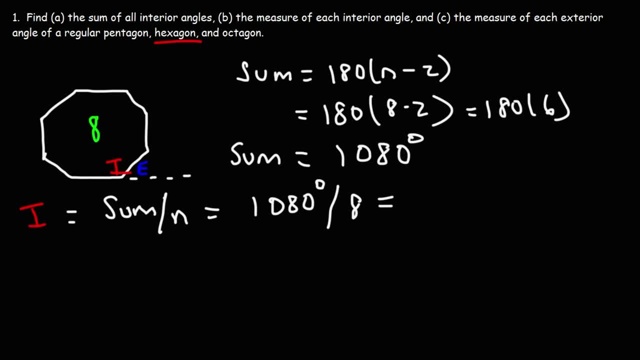 So the measure of each interior angle is 135.. Now let's calculate the measure of each exterior angle. So it's simply the complement of the interior angle, So 180 minus 135. That is going to be 45. And then, to confirm it, it's also 360 over n. 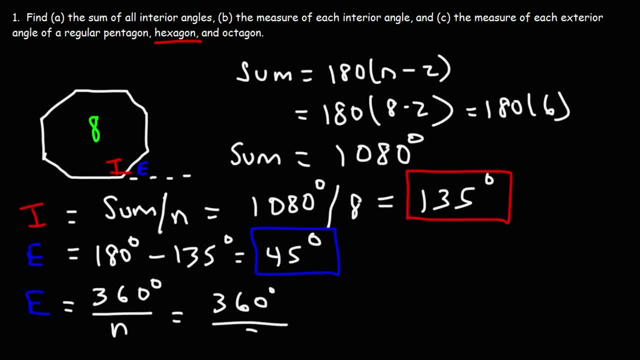 So if we take 360 degrees and divide it by the eight sides- and this we can probably do mentally, So I'm going to break this up into 320 and 40, and then divide each by 8.. 32 divided by 8 is 4.. 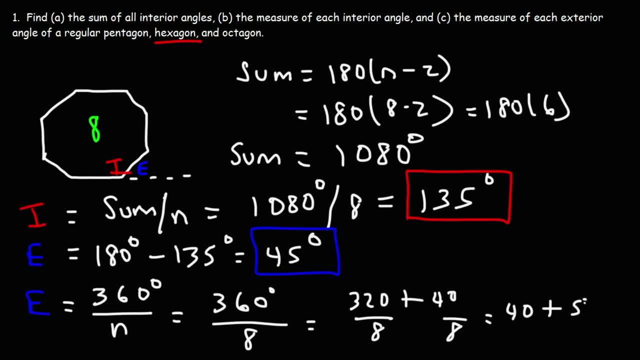 Add the 0,, you get 40.. 40 divided by 8 is 5.. So we get the same answer of 45 degrees. So now you know how to calculate the sum of all of the interior angles of a regular polygon. 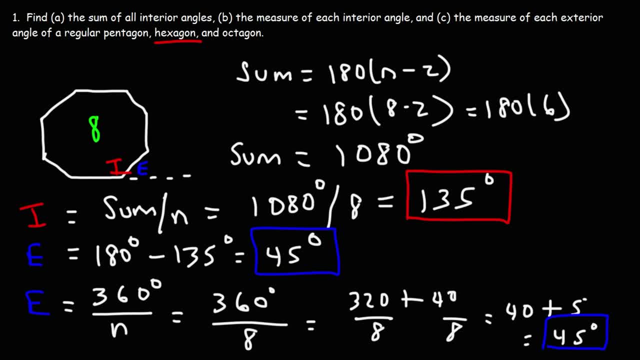 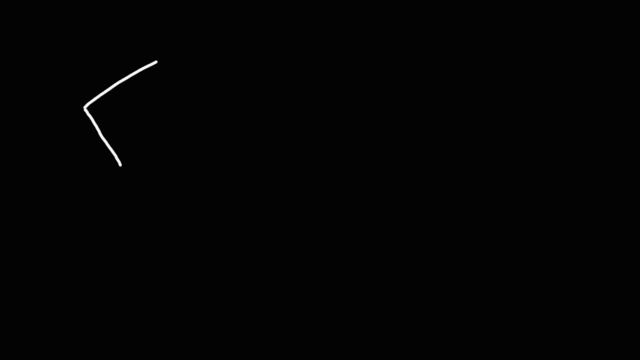 You know how to find the measure of each interior angle, as well as the measure of each exterior angle. Now let's go back to the regular pentagon. Let's talk about why the measure of each. Let's talk about why the measure of each. 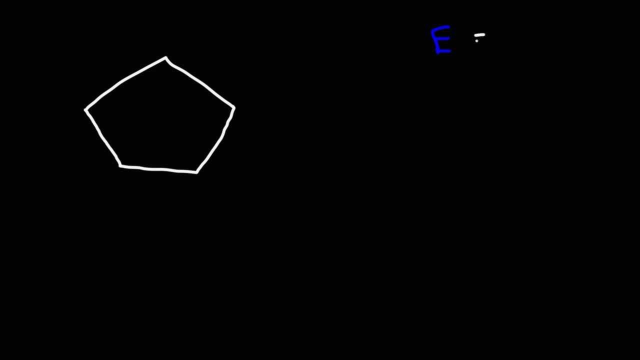 Let's talk about why. the measure of each, Each exterior angle is simply 360 divided by n. 360 is the measure of a full circle, And if we divide it by the number of sides of a polygon, we get the measure of each exterior angle. 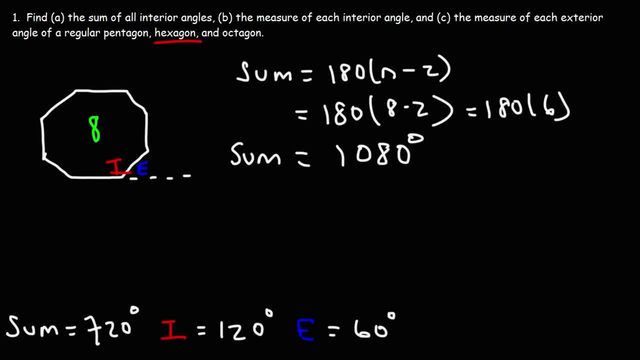 Now to calculate the measure of each interior angle. It's going to be the sum divided by n, So that's 1080 degrees divided by the 8 sides, So the measure of each interior angle is 135.. Now let's calculate the measure of each exterior angle. 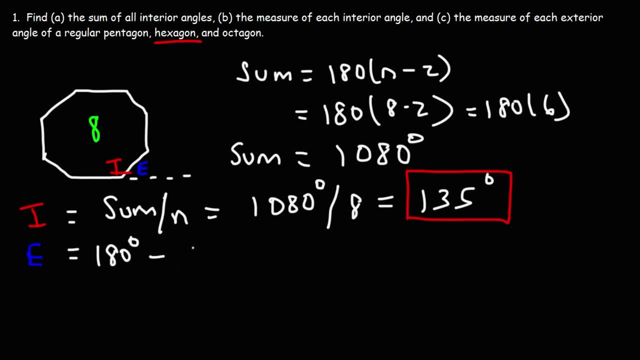 So it's simply the complement of the interior angle, So 180 minus 135.. That is going to be 45.. And then, to confirm it, It's also 360 over n. So if we take 360 degrees and divide it by the 8 sides, 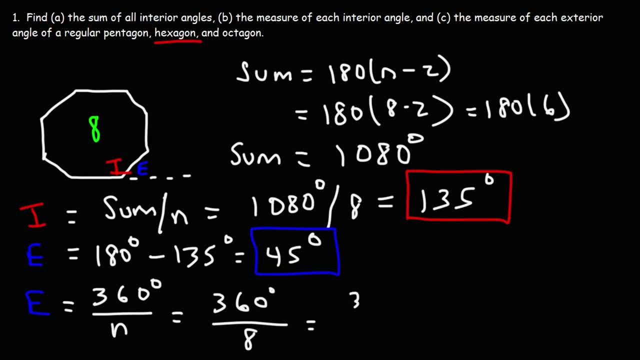 And this we can probably do mentally. So I'm going to break this up into 320 and 40. And then divide each by 8.. 32 divided by 8 is 4.. Add the 0,, you get 40.. 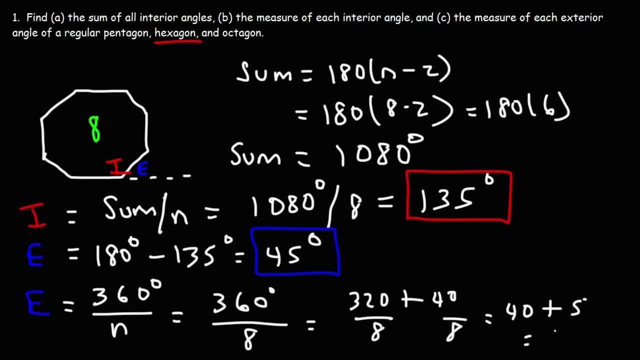 40 divided by 8 is 5.. So we get the same answer of 45 degrees. So now you know how to calculate the sum of all of the interior angles of a regular polygon. You know how to find the measure of each interior angle. 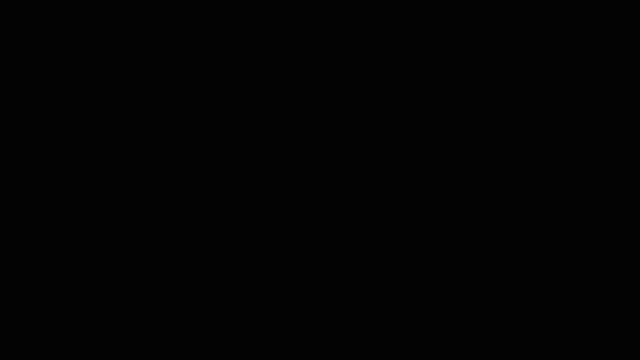 As well as the measure of each exterior angle. Now let's go back to the regular pentagon. Let's talk about why the measure of each exterior angle Is simply 360 divided by n. 360 is the measure of a full circle. 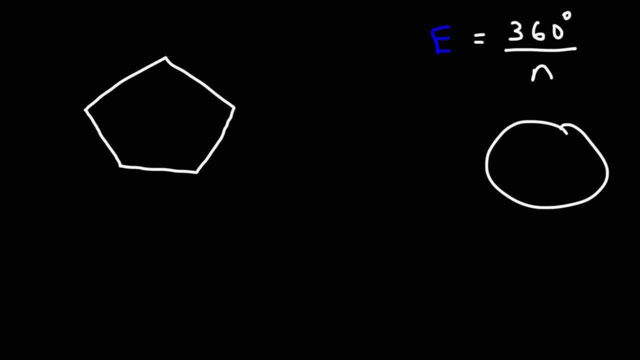 And if we divide it by the number of sides of a polygon, We get the measure of each exterior angle. Let's understand why. First let me draw a better polygon And you can depend on Again. So we have to add all of the height of the rectangle. 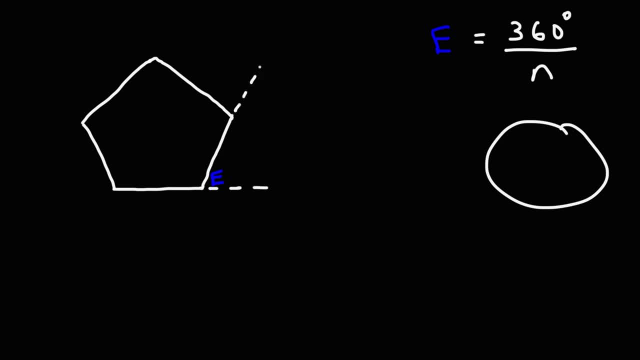 And we can subtract the square. So we have now object Disneyland DE DENIS, I'm going to add. Here's the next one. So those are the five exterior angles, if we draw it in a counterclockwise direction. 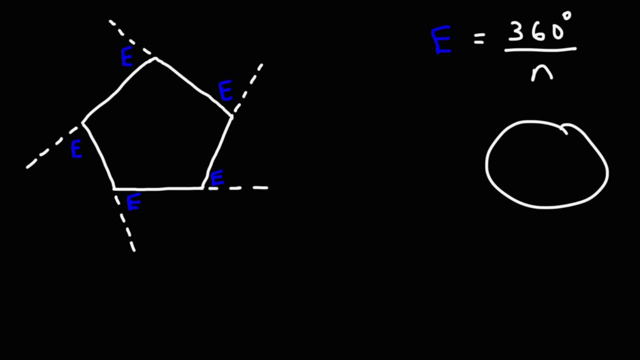 So now let's draw the arcs. I'm going to color code them. So this is the first arc drawn in a counterclockwise direction. Okay, Okay, This is the second arc. This one is the third, Fourth, Fifth. 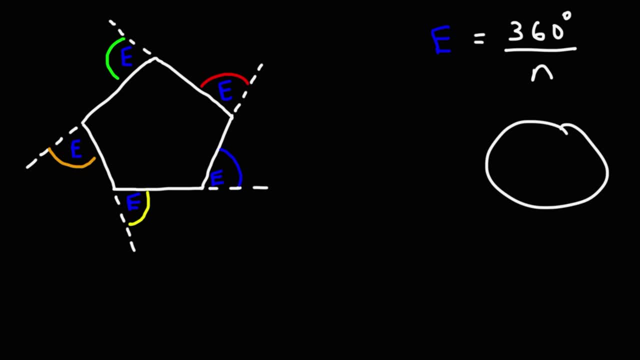 Notice that if you put all these arcs together they form a circle. So here's the first one in blue, Here's the second one in red, And then here's the third one in green, The fourth one in orange. 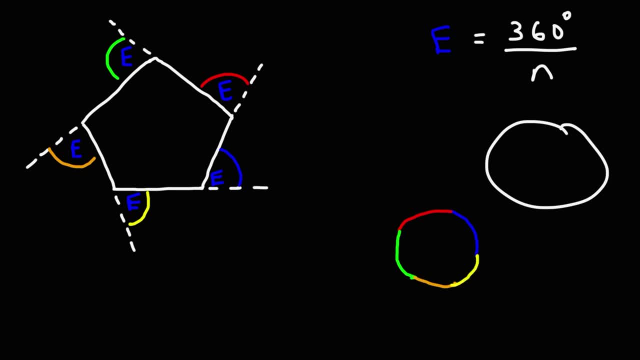 And the last one in yellow. So you can see that these five exterior angles, they form a circle with a total angle of 360 degrees. So if you divide them by the number of exterior angles, which is the same as the number of 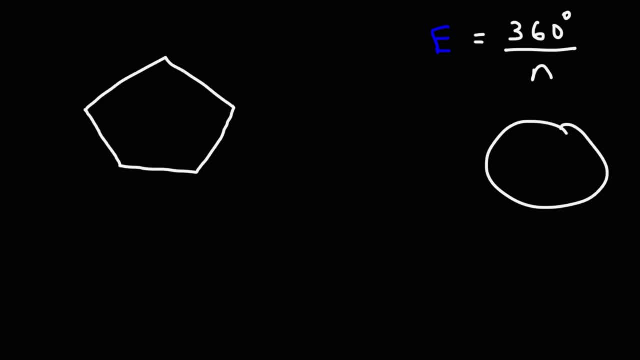 Let's understand why. First let me draw a better polygon. Now let's draw each exterior angle. So this is one exterior angle. Actually, I already used that line, so now I have to use a different one. So let's start with the exterior angle. 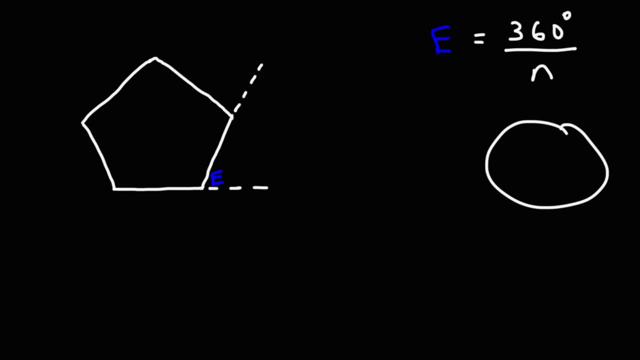 Draw a dollar thingy. Let's draw a dollar thing. Let's draw a dollar thingy. Here's the next one. Add a dollar thing to the continue link, Thank you. So those are the five exterior angles if we draw it in a counterclockwise direction. 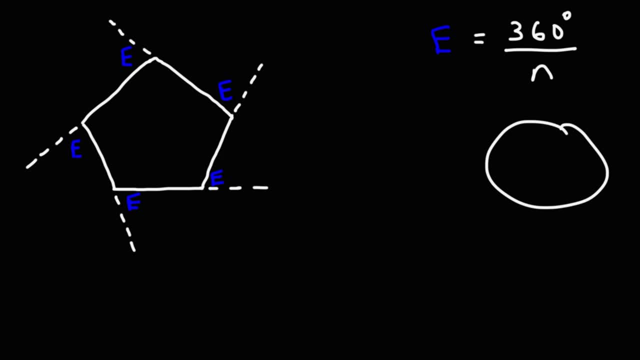 So now let's draw the arcs. I'm going to color code them. So this is the first arc drawn in a counterclockwise direction. This is the second arc. This one is the third, Fourth, Fifth. Notice that if you put all these arcs together, they form a circle. 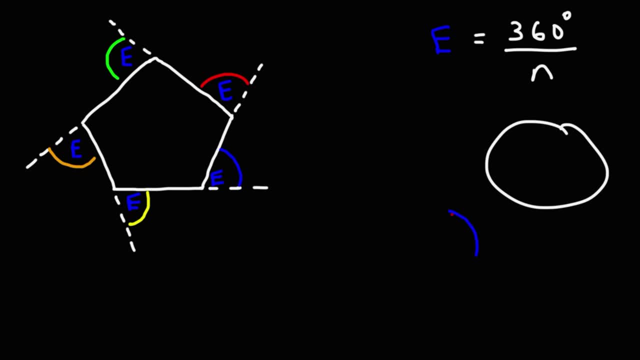 So here's the first one in blue, Here's the second one in red, And then here's the third one in green, The fourth one in orange And the last one in blue And the last one in yellow. So you can see that these five exterior angles, they form a circle with a total angle of 360 degrees. 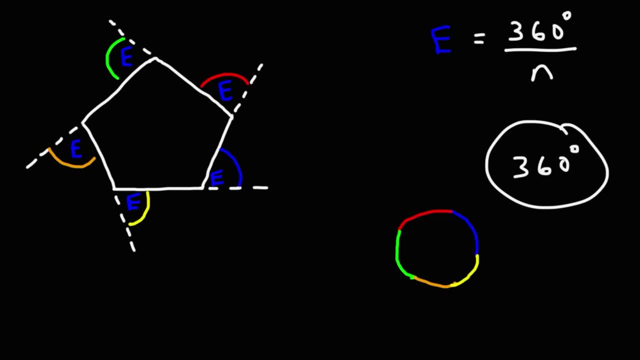 So if you divide them by the number of exterior angles, which is the same as the number of sides of a polygon, that's going to give you the measure of each exterior angle. So by drawing it you can see that those five arcs, they form a shape of a circle.